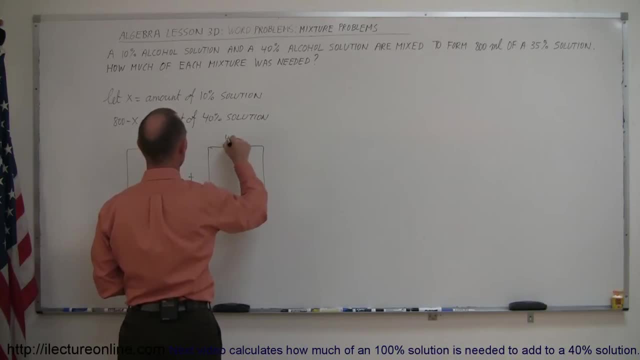 of alcohol that we got And the 40% solution. so 40% right here And that equals the final solution that we have. That's equal to a 35% solution. All right, now I'm trying to keep track of the alcohol And how. 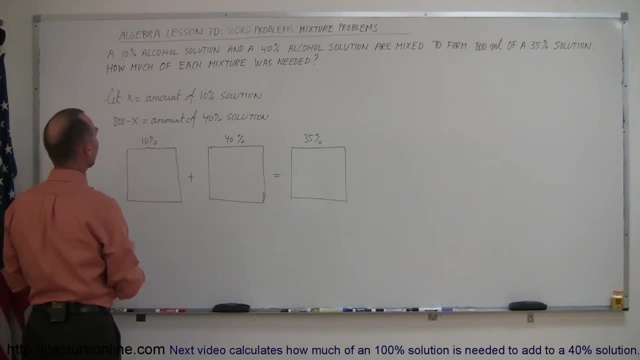 much alcohol was there in the 10% solution. Well, I multiplied the amount of that solution times the percentage of the solution, So 10% multiplied times the amount that I have. So this represents, away from the 10% amount there, Then from 75%, the amount of alcohol that I have in my 10% solution. 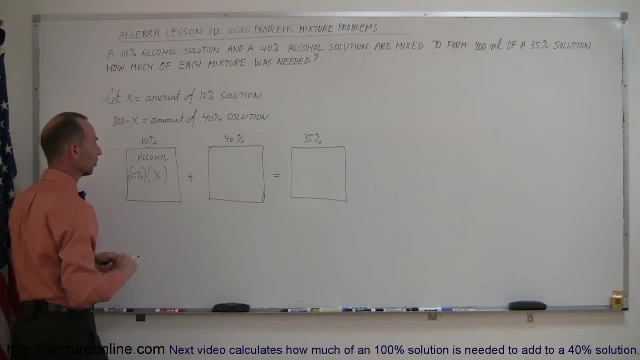 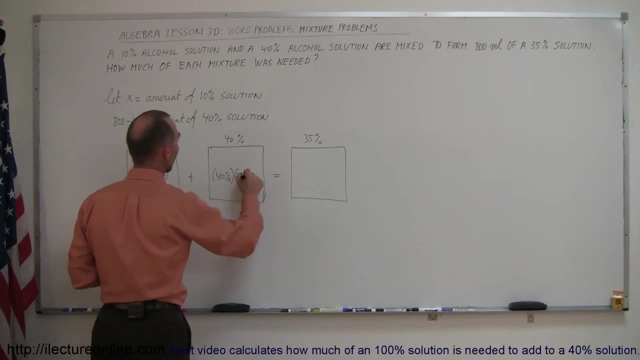 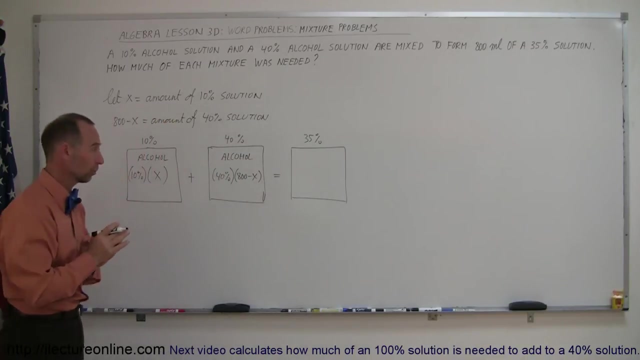 So 10% times the number of milliliters of that solution. Here I multiply the percentage of alcohol in that solution times the amount that I got. This is 800 minus x. This represents the number of alcohol that I had from the 40% solution. So the amount of alcohol that 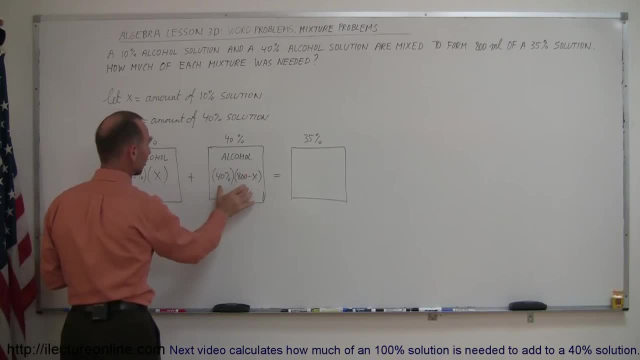 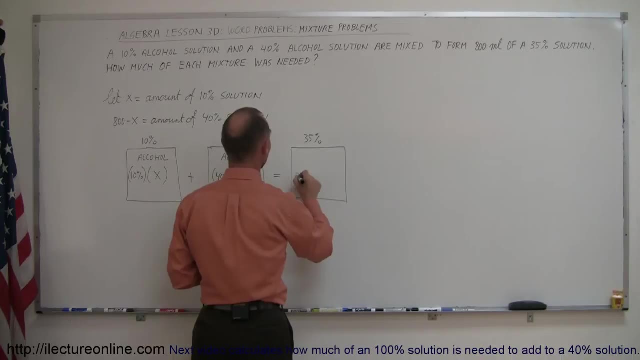 I have from the 10% solution. The amount of alcohol that I have from the 40% solution must equal- Okay, i have in my final solution. so that would be 35 solution times the total that i have. in that case i have 800 milliliters and that would be the alcohol that i have in my total solution. that's. 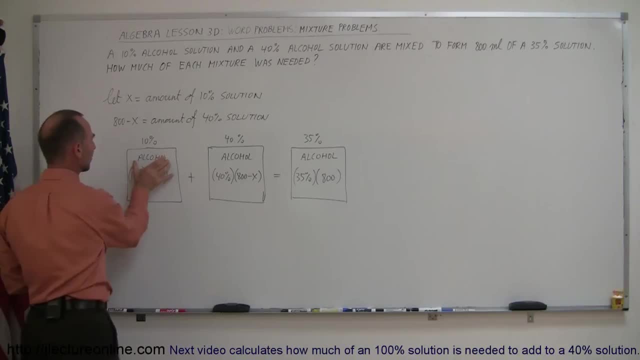 the best way to set up the equation. so the amount of alcohol in my 10 solution plus the amount of alcohol my 40 solution equals the amount of alcohol in my 35 solution, and by multiplying the percent alcohol in the solution times how much of the solution i use, that then gives me. 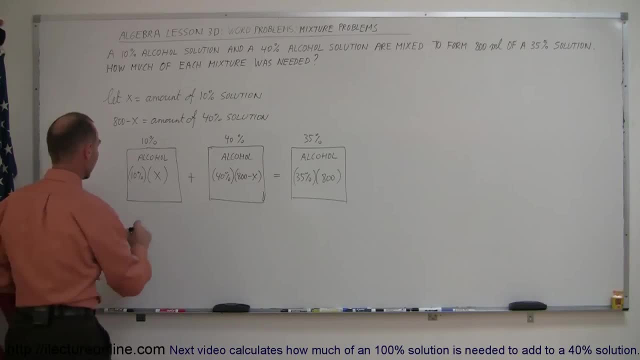 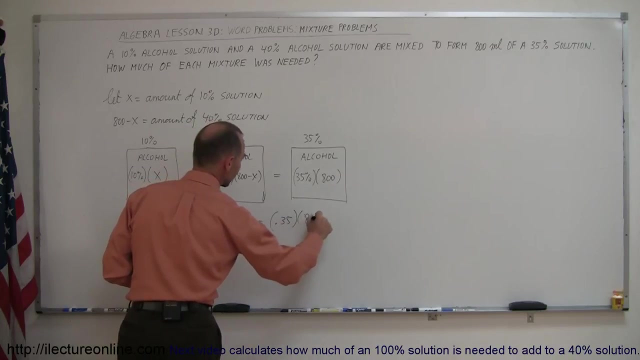 the alcohol in that solution and now i have an equation. so 0.1 times x plus 0.4 times 800, minus x equals 0.35 times 800.. now i have to solve that for x. first thing i want to do is get rid of. 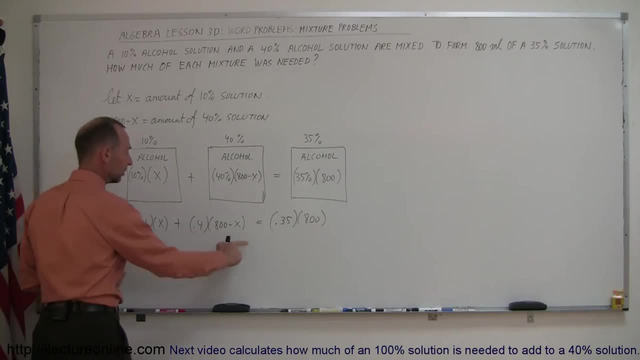 decimal places. i have one decimal place here, one decimal place here here, two decimal place there. that means i multiply both sides equation by a hundred to get rid of all the decimals. so multiply the left by a hundred and multiply the right by a hundred. okay, a hundred times point one gives me ten, so it gives me ten times x plus. 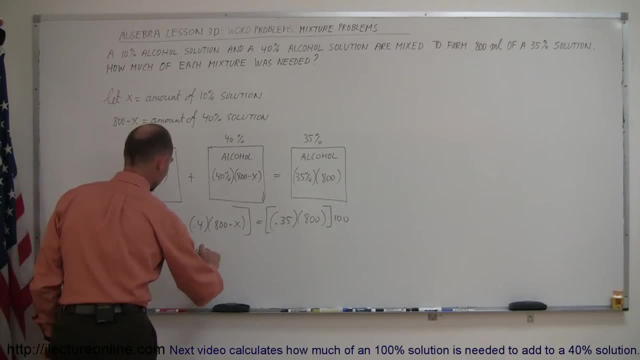 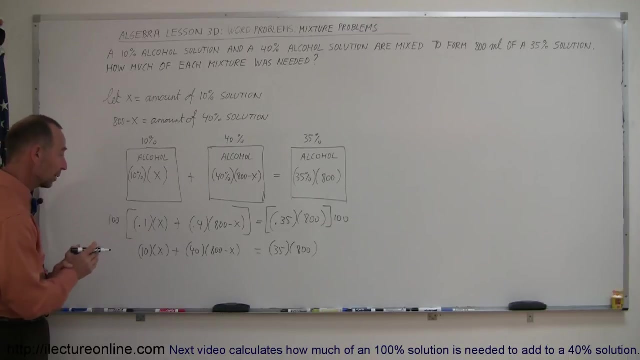 a hundred times point four gives me forty. so that is forty times eight hundred minus x, and that equals a hundred times point three. five thirty five times eight hundred. all right, next i go ahead and multiply everything out to get rid of parentheses, so this gives me 10x plus 40 times 800. that's 32 000 minus 40 x equals. 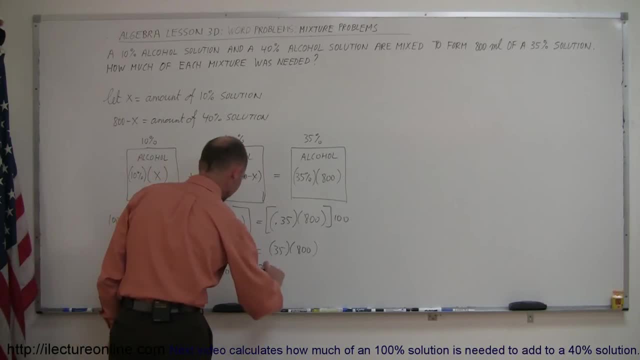 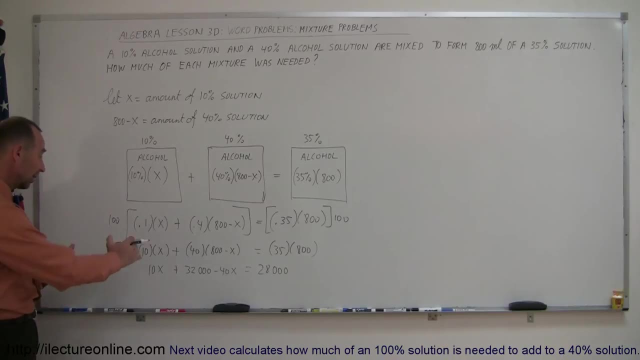 and 35 times that, that's 24, that's 28 000.. all right. next step is to move all the x's to one side, and they're already on the left side, so i move those, and then i move all the numbers to the other side, so i need to move the 32 000 to the 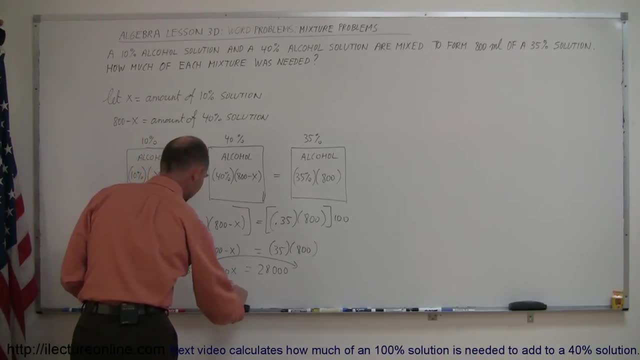 right. so i get 10x minus 40x. on the left side equals 28 000 minus 32 000.. okay, at this stage i can go ahead and combine like terms. i can add the left, add the right. let me move over here. 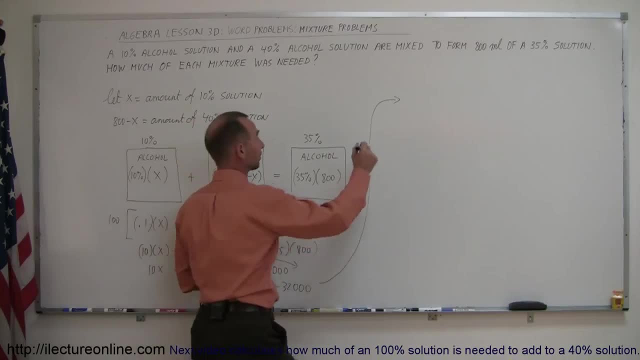 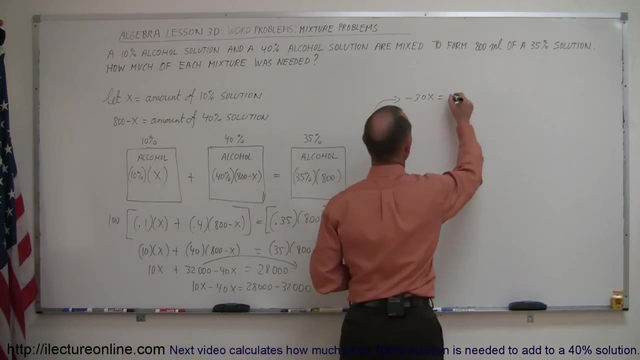 and do that, so 10x minus 40x, that's minus 30x, equals 000, that's minus 4 000.. and then i go ahead and divide both sides of the equation by minus 30, so that cancels out and 0 and 0 cancels out, and so x is equal to. hmm, that doesn't give. 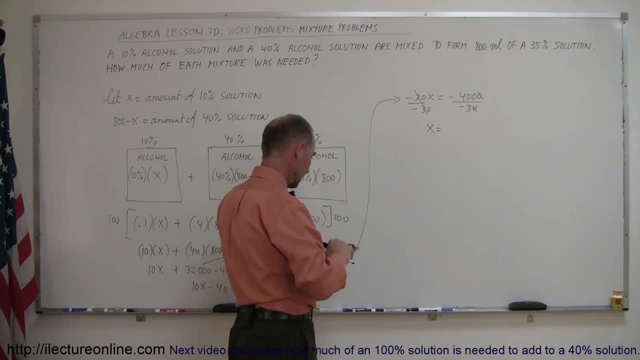 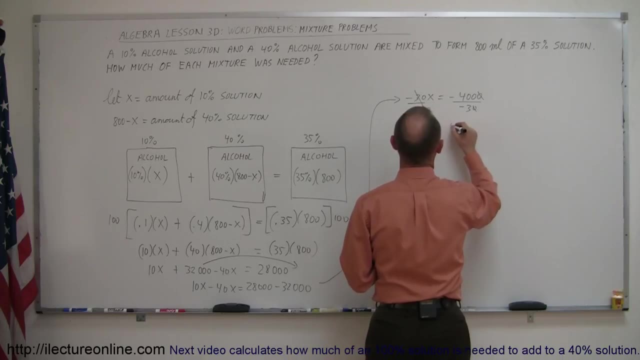 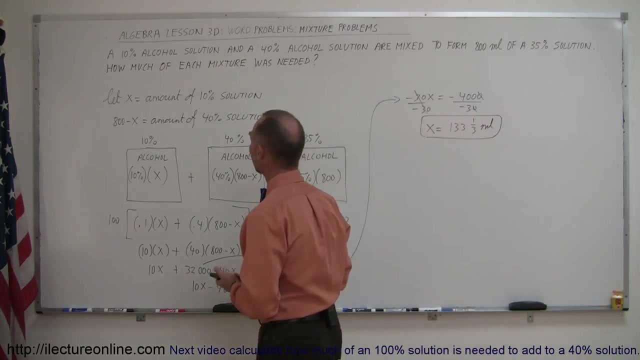 me. a nice round number does it well: 400 divided by 3 is 133 and a third. so this is equal to 133 and a third milliliters. okay, come back over here. so how much of the 10 solution do i need? i need? 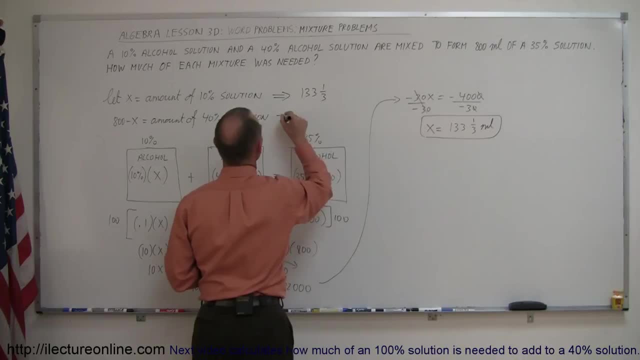 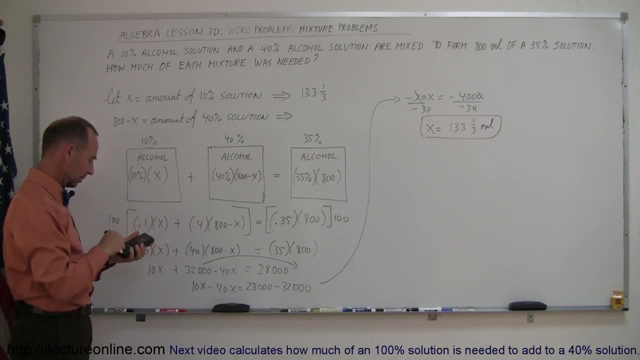 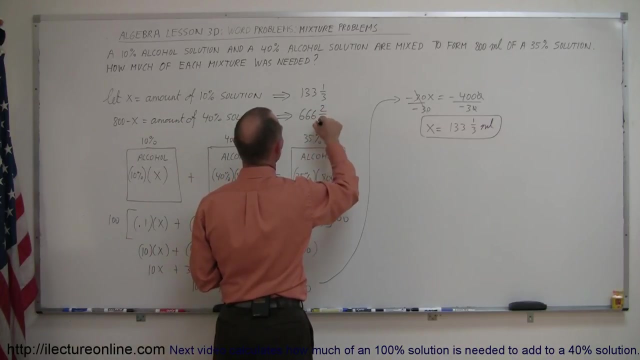 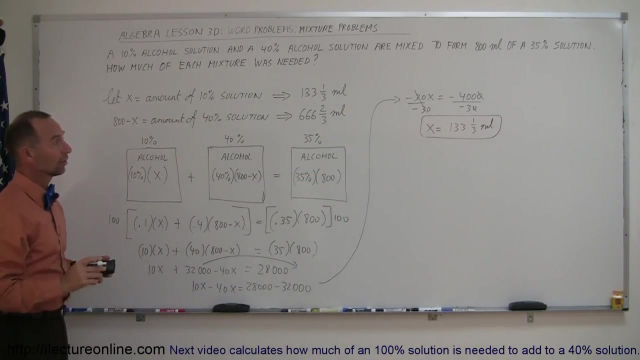 133 and a third milliliters. so how much do i need of the 40 solution? well, 800 minus 133 and a third, that's 666 and two-thirds of that solution. so that would be the number milliliters, number of milliliters, that solution, and that's how you find the answer to this particular problem. all right.